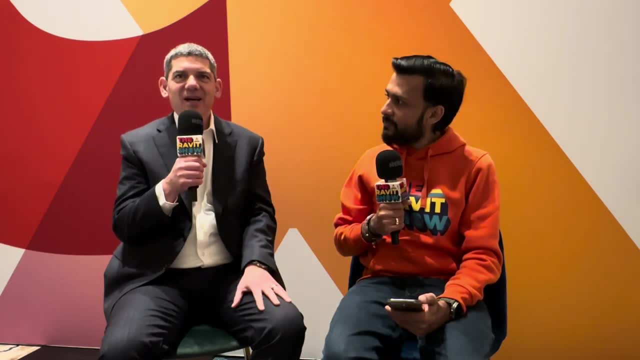 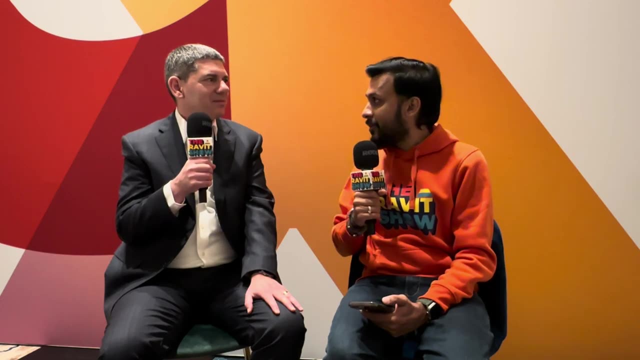 And that gives us the capabilities that developers need to be successful in building these Gen AI apps. Okay, That's pretty interesting Great insights there. I also when I was reading your blog. obviously, you mentioned a little about the challenges as well. When you kind of you know, when you're developing the AI assisted capabilities for databases, there are a lot of challenges. How did the team overcome those types of challenges? Would you like to share a little? 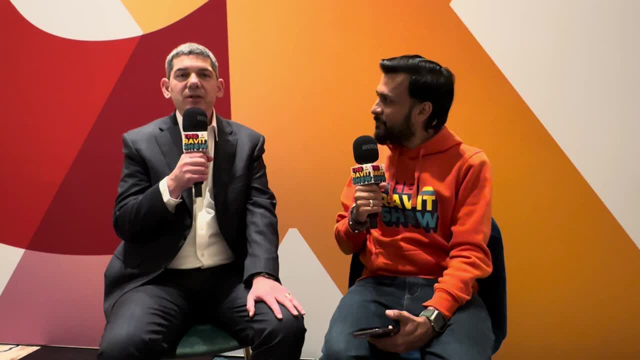 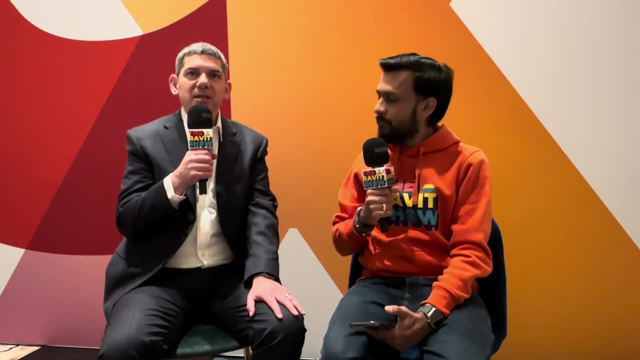 Yeah, that's a great question And, you know, let me distinguish between two things. One is: how do we bring Gen AI features up to speed into databases that help developers build Gen AI apps? That is category number one, which I kind of referred to before. 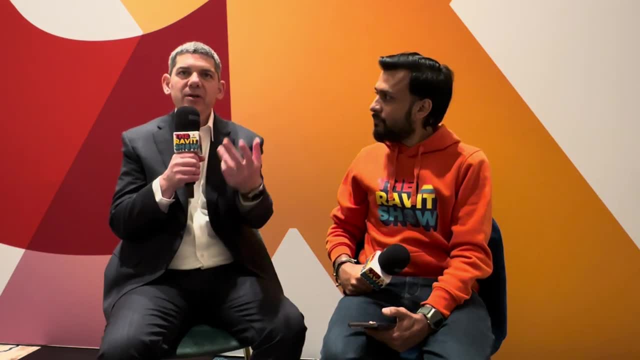 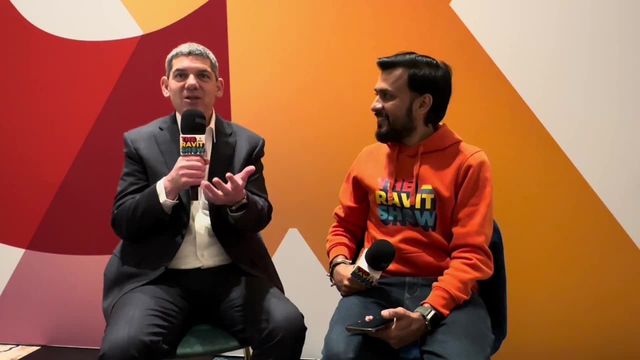 The second one which I think you're asking about is: how are we using Gen AI to make the lives of developers and operators easier? True, And I think on the second one is we just launched Gemini in databases yesterday. We're super excited about it. 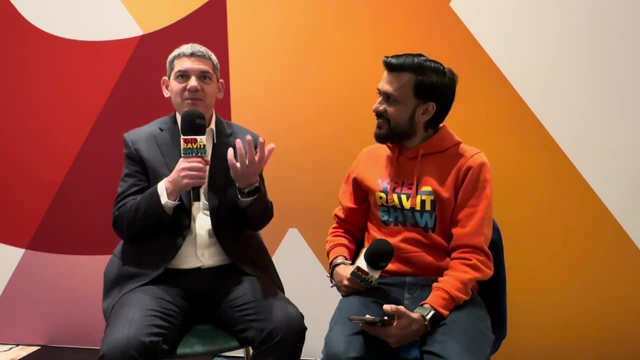 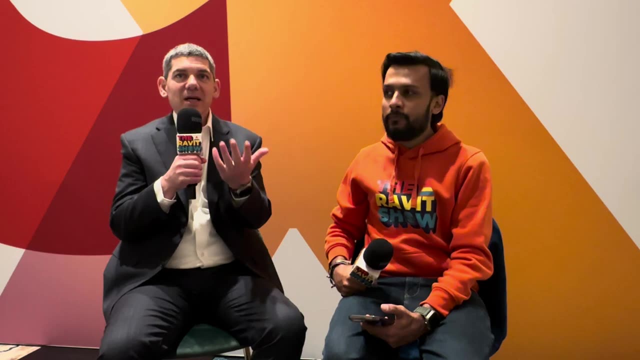 We're at it as three key pillars in what we announced. The first one is how do we help developers kind of use natural language to generate SQL, So really help developer productivity? The second one is how do we help migrating applications from legacy databases to more modern databases? 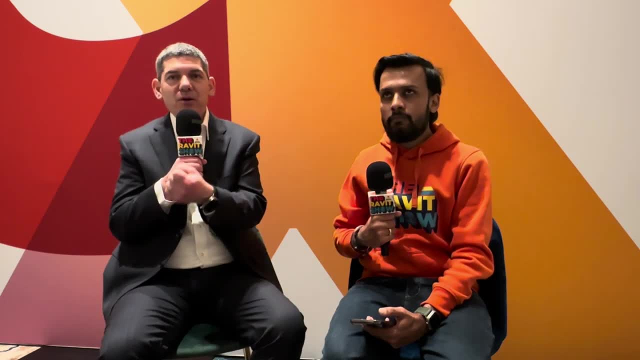 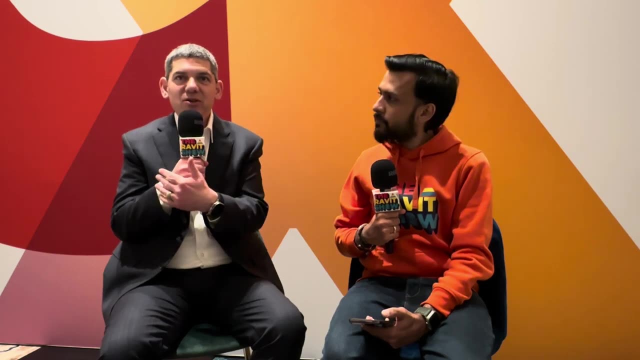 like Postgres and how can we use Gen AI for that? The third one is the piece that really is most exciting to me personally, which is how are we using Gen AI to help customers manage your entire database estate Right Really have like this AI system, DBA? 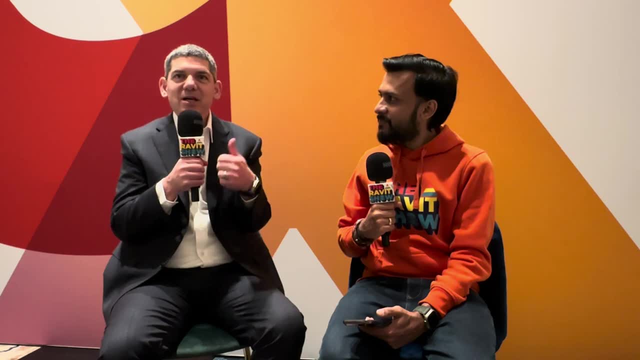 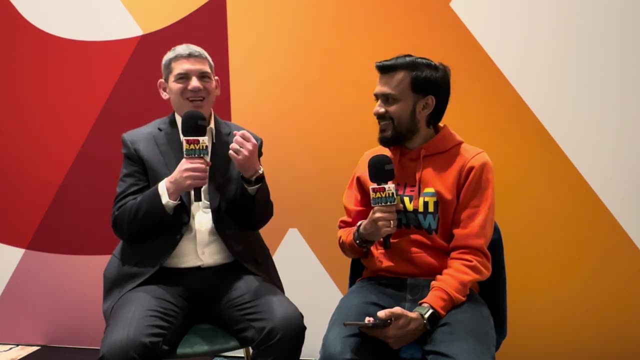 that sits side by side with them and can help on performance management, security governance. By the way, when you go to sleep, you know the AI system is still at work for you and watching your systems, And so we really have driven a lot of innovation. 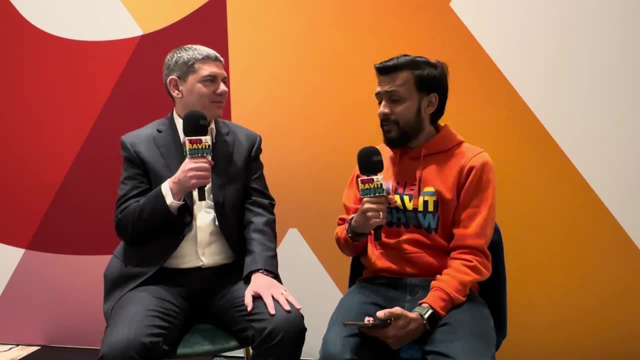 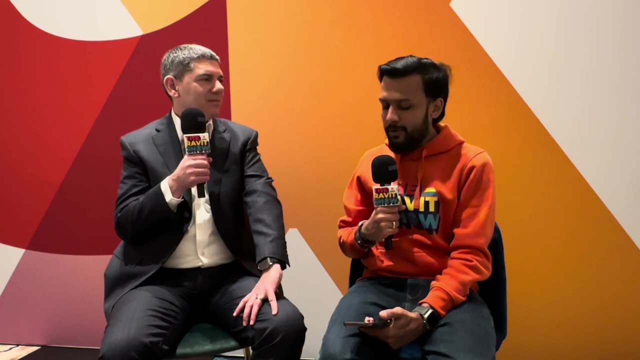 and customers are super excited about that. Yeah, that's pretty good for sure. In terms of, you know, I also saw the introduction of Alloy DBA AI. What new opportunities do you see for developers creating Gen AI around that side? Would you like to share a little? Yeah, that's a great question, You know, for those who are not, you know, aware of Alloy DB. Alloy DB is a Postgres compatible engine, but really meant for, you know, the most demanding workload. So it's more scalable, more performance. 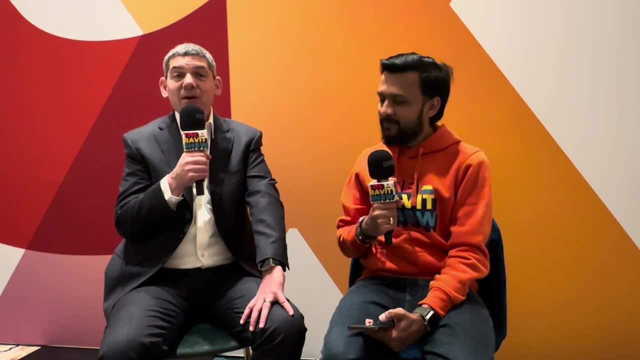 easier to manage than standard Postgres And, by the way, we also have Alloy DB Omni which you can run anywhere. So we will support this not only on GCP, but also on other clouds, also on premises, And so it truly gives customers a one-stop shop. 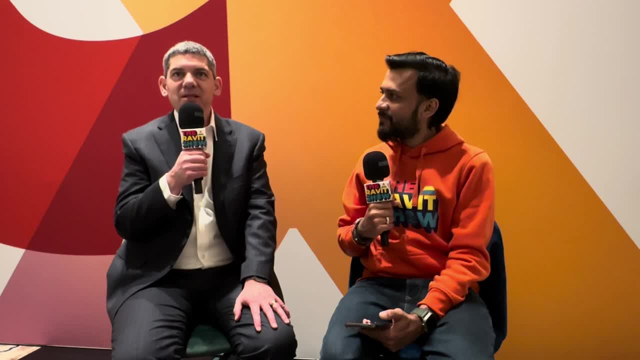 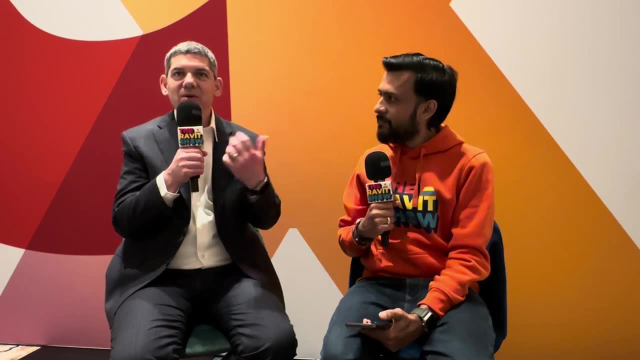 you know, for all their database needs, no matter where they want to run or modernize. Now, part of Alloy DB is we have a set of features we call Alloy DBA AI, which are features that really help developers as they're building Gen AI apps. We announced that last year And then yesterday we announced a huge step up in capabilities around Alloy DBA AI. So just to summarize a few of those one is we announced a new vector search capability that is PG vector compatible but is built on technology that we've built and developed. 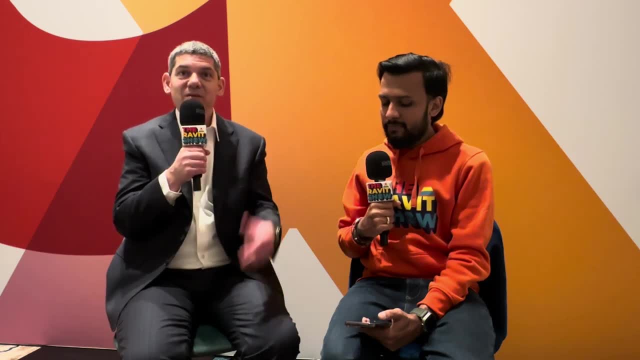 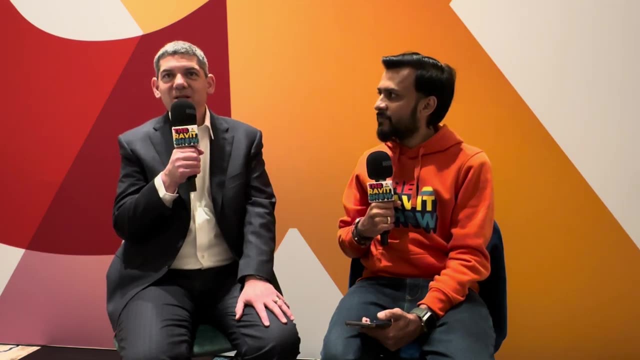 inside of Google for the last 12 years for supporting, you know, some of our businesses like ads and YouTube. We're using that technology now to deliver very differentiated vector search capabilities within Alloy DBA AI. So that, I would say, is announcement number one. 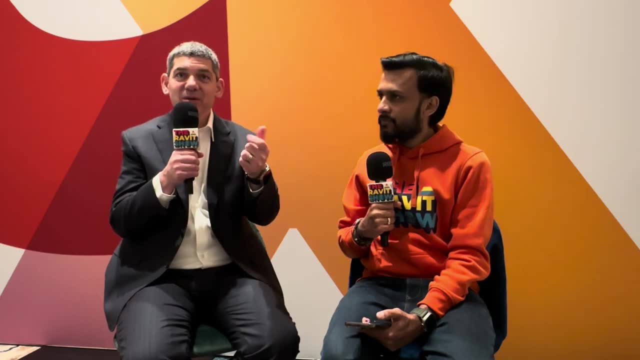 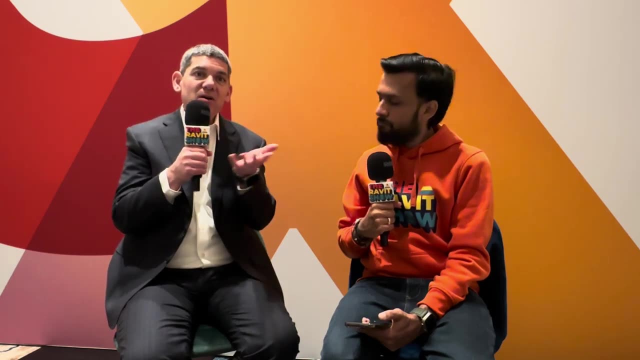 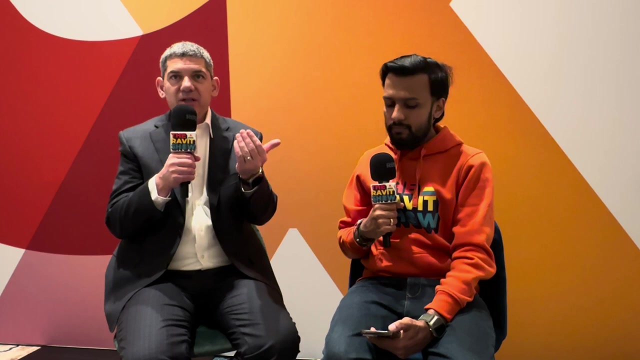 Number two is we announced natural language interface to Alloy DB that helps developers build applications that take natural language prompts. Now you could kind of say like hey, okay, but everyone's doing that. The problem, though, is truly creating natural language interface. 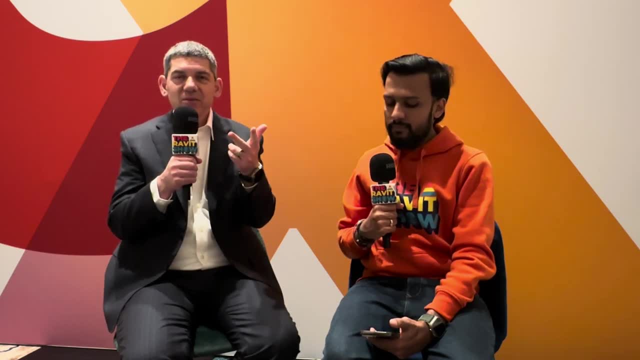 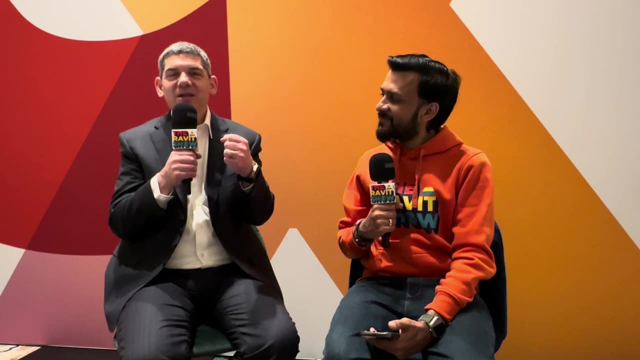 that is very accurate, very secure and very flexible is actually incredibly hard and no one has really done a great job at that. So we've taken this on. We're building that into the database. We've added new security capabilities also in the database. 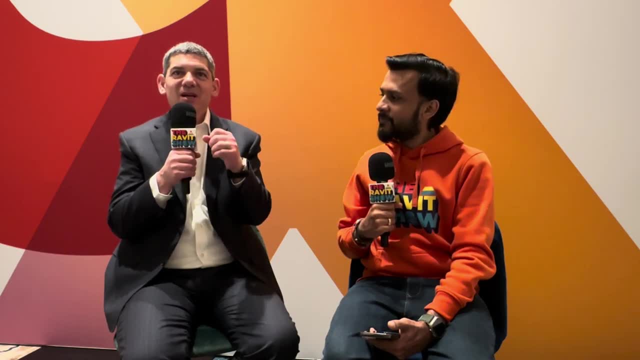 to not only make this flexible and accurate, but also secure, And so we do believe, you know, Alloy DB is really charting a new course for databases in this space. And then the third thing we announced yesterday around Alloy DBA, AI is remote model management. 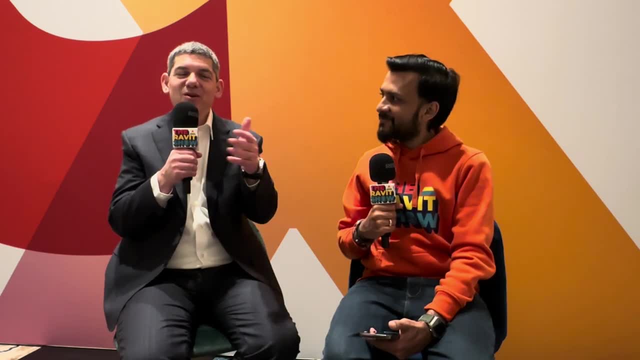 meaning today already Alloy DB can call vertex AI- you know from within transactions- And, for example, if you want to generate embeddings or do an inferencing. So we've expanded that now to also include other providers. You can also connect Alloy DB with Hugging Face. 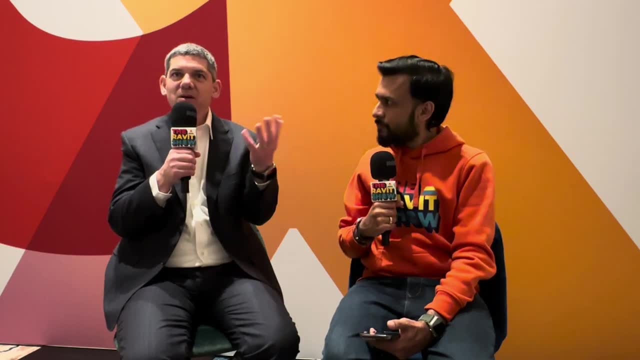 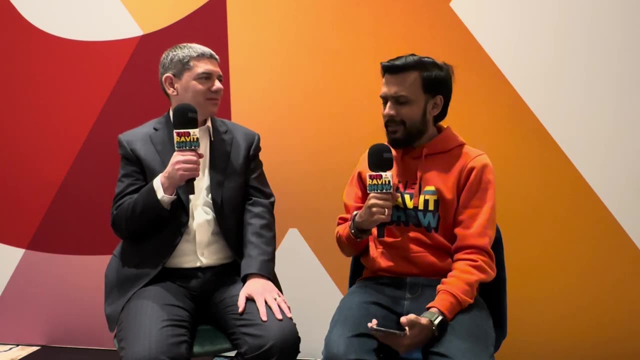 with Anthropic. We even support open AI as part of that. So you know we're really driving this to be. an open ecosystem, runs anywhere, connects to any other AI service. Sounds great, Great insights and such great integrations for sure. 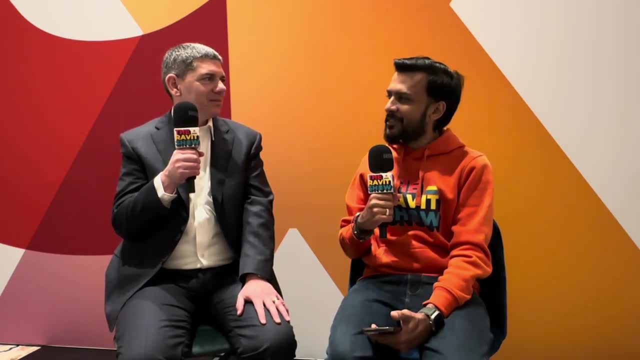 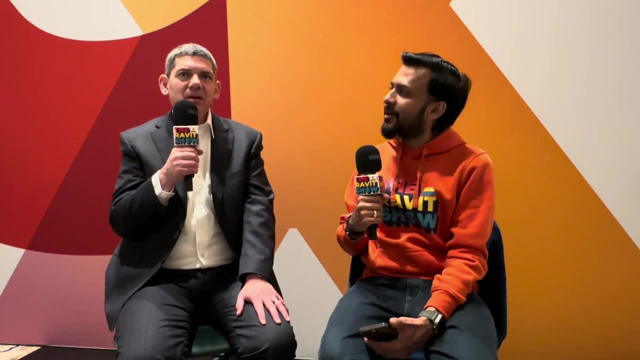 Thanks for sharing that, Andy, Quickly, in terms of: do you have any use cases that you would also like to share with our audience? Obviously, YouTube, Google Search. you know these are fantastic, But any other use case that comes to your mind? 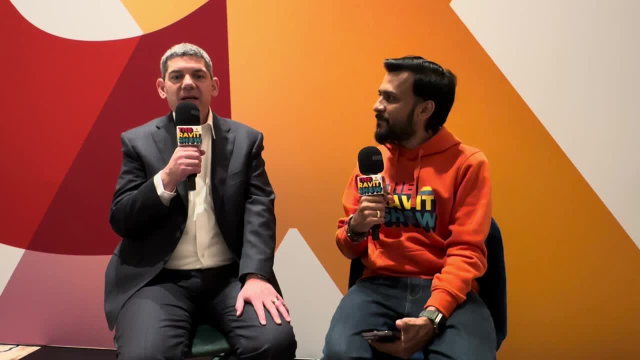 Yeah, absolutely So. we have, you know, some really great case studies. We have a company called Regnology. They're in the compliance regulatory space, Serve a lot of financial services. They have a chat bot that they've built on top of Alloy DB AI. 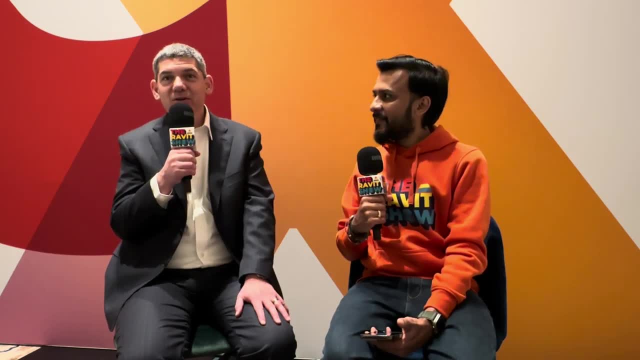 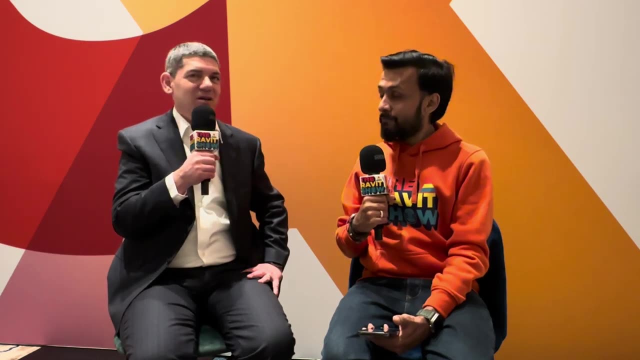 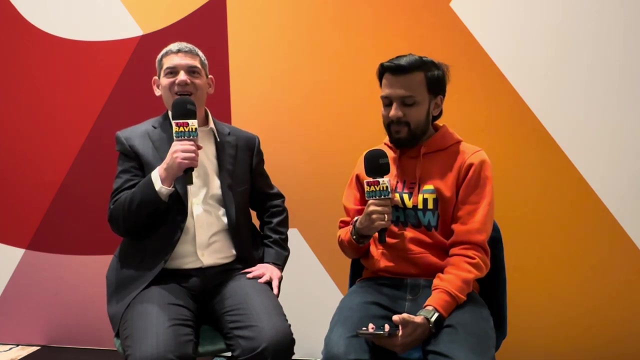 To basically enable both external customers and their internal employees to ask regulatory inquiries, And so that's made them way, way more efficient and has really delivered a lot of value to customers. You know a company called Linear that is in the developer space. 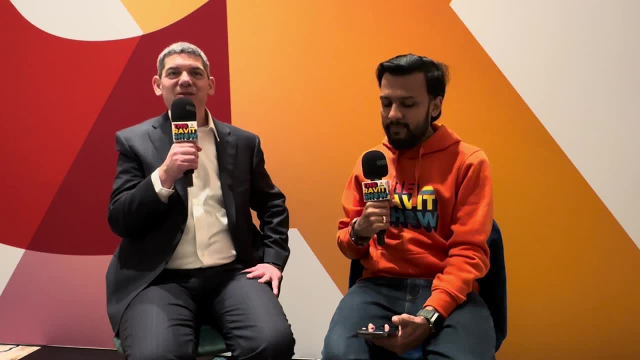 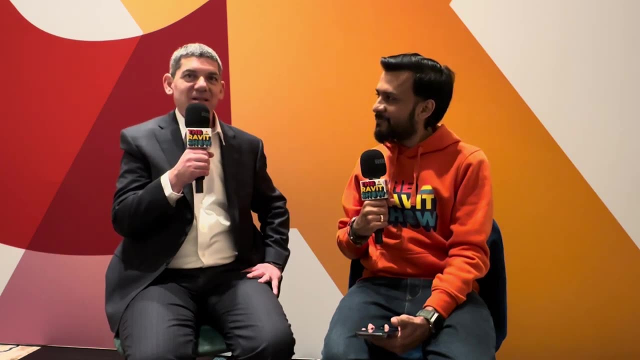 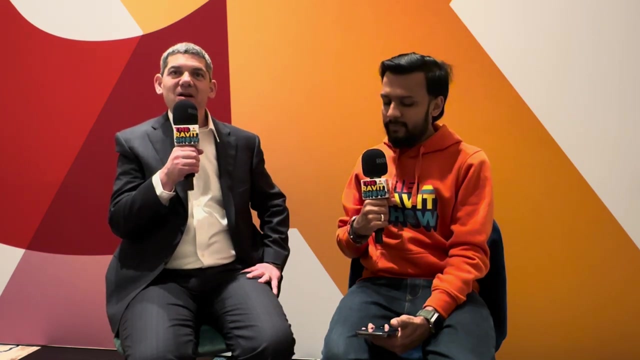 are also using Alloy DB AI to do similarity search between support tickets, making it much easier to detect- you know, when you have duplicate support tickets coming in, Yeah Right, And making the support organization more effective. So we're seeing a lot of these use cases. 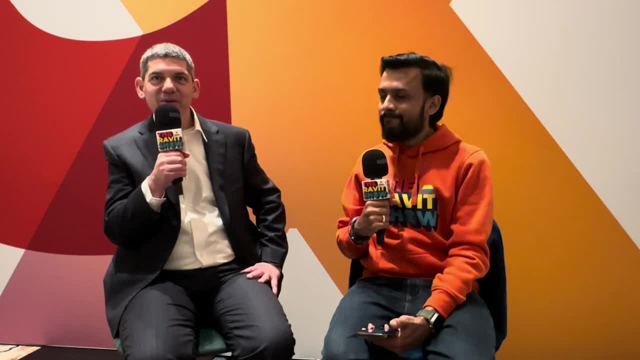 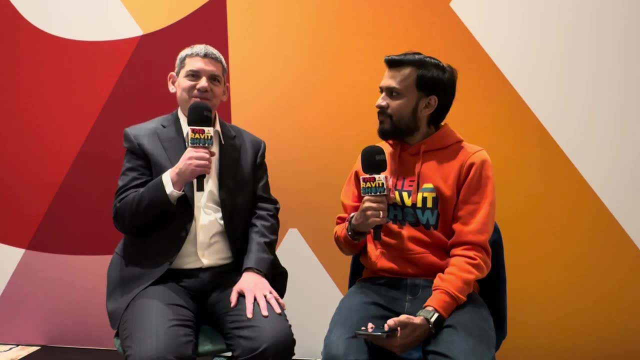 where both either internal employee productivity is being helped and supported or external customer experiences are getting better And in some cases, like Regnology, both of those. That's fantastic. Thanks for sharing that example in the use case as well, But in your. just because we are on this topic, 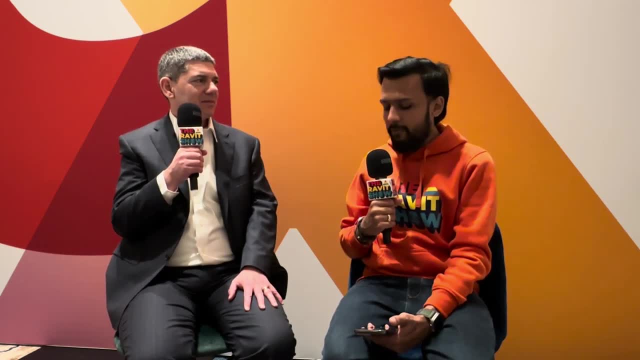 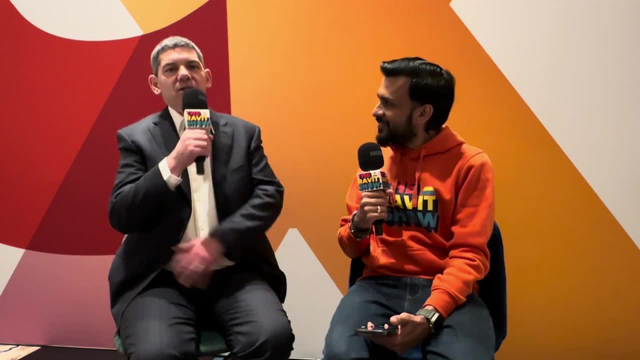 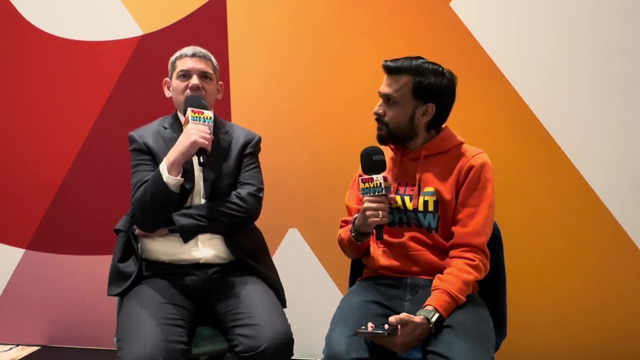 data in terms of the business transformation. Do you have any other thoughts? That's a great question, You know. I think what's been really exciting about bringing these vector capabilities into the operational databases that customers are already using is that they don't have to spend a lot of time right. 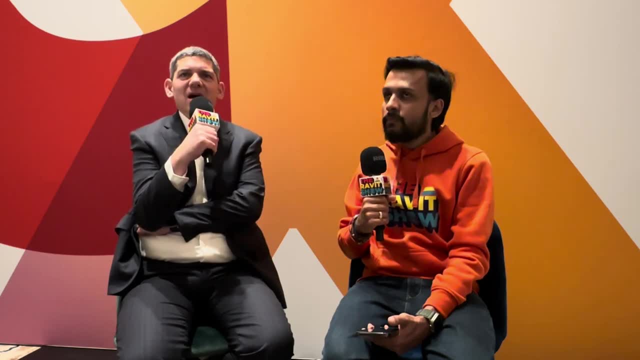 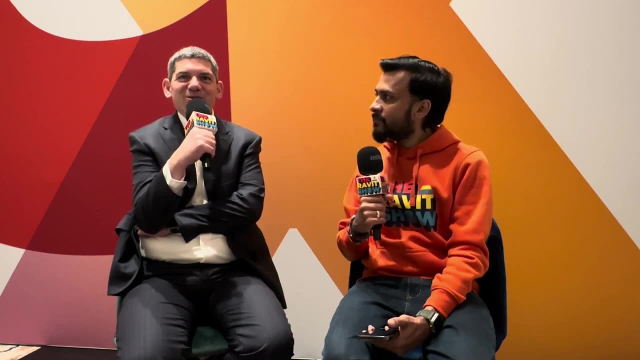 figuring out how to use a new database, moving data around like a lot of complexity. right In this world. they can actually just focus on building their Gen AI feature. right, You have their existing database. the data is there. vector capabilities come in. 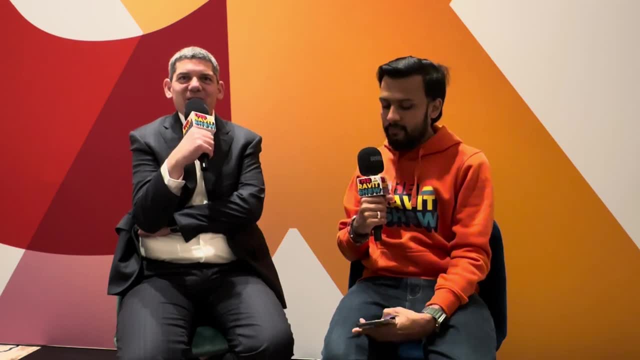 they can still use standard SQL that they're used to to basically query the database. So I'd say the big impact has really been productivity and simplicity, and so we are very committed to really bring these kind of capabilities to all of our databases so that customers can actually 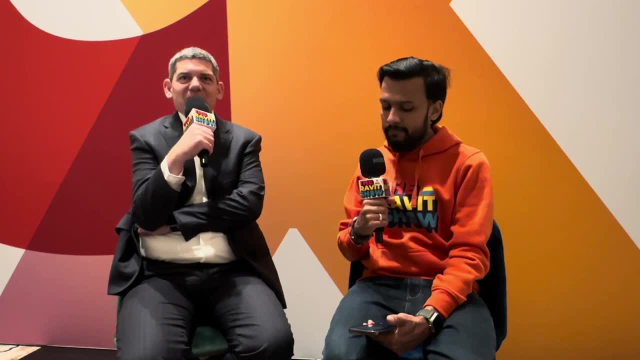 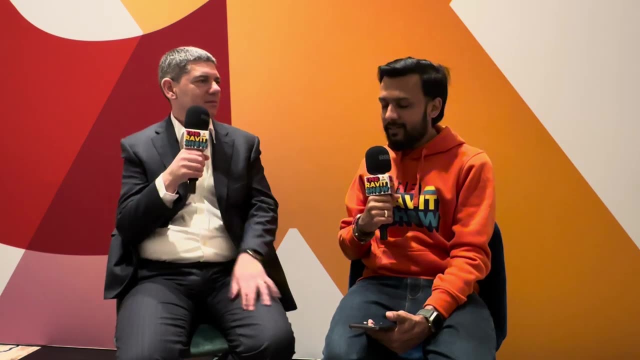 just use the systems they're already used to using and love, as opposed to having to try and figure out how to build new pipelines and kind of add complexity to their systems. Yeah, I think that makes a lot of sense In terms of also looking forward and ahead in the game. 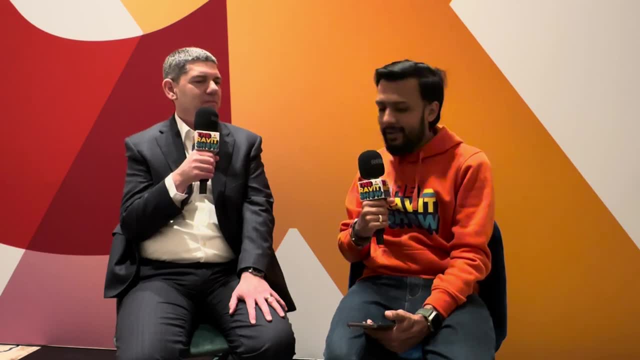 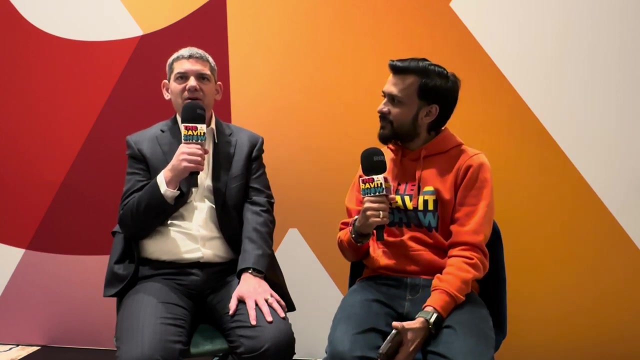 what are the next big steps for Google Cloud in advancing in AI and in advancing in AI capabilities and also the database services? Any thoughts? Yeah, that's a great question. I think one of the things that really differentiates us at Google is that AI is truly part of how we think. 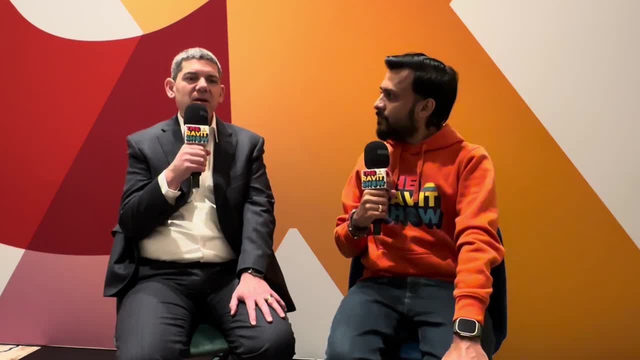 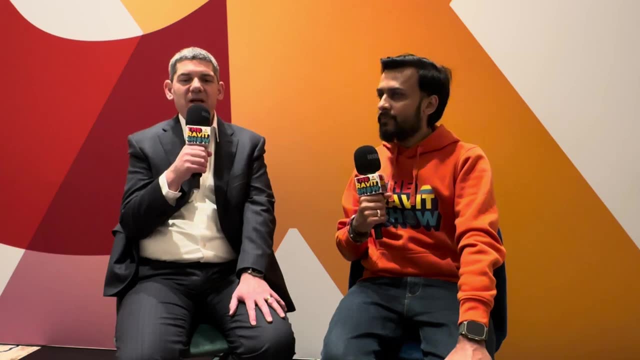 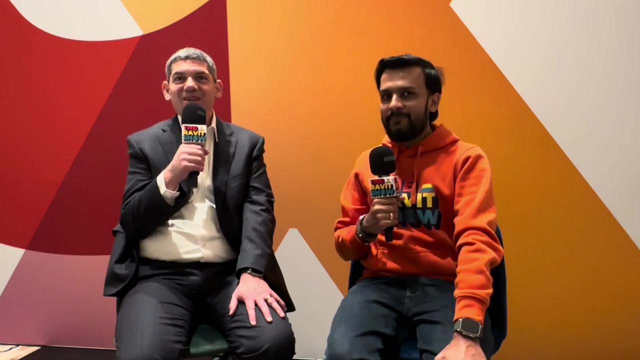 about the company and how we operate. And we're actually the only provider that both has- you know, its own hardware infrastructure, right to train and inference models, And then we're also the only ones who really are training. you know, only hyperscaler, really, that's training at scale. 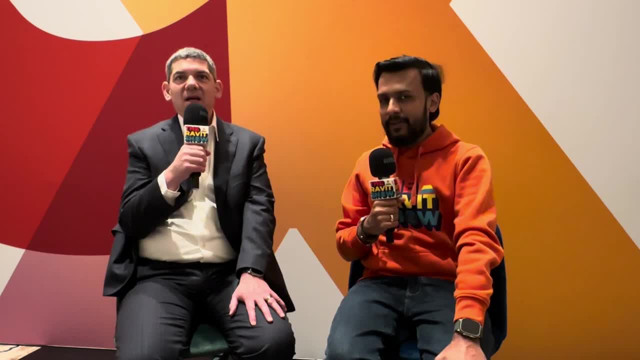 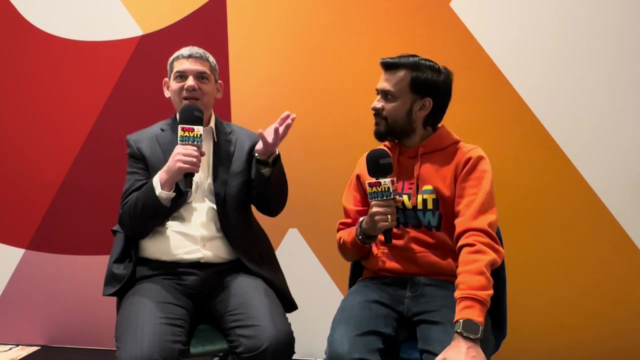 right and not just using third parties for that Right. What that actually gives us is a real opportunity to innovate more quickly for our customers. So, for example, as my team is working on natural language to SQL translation, my team can actually upstream data sets. 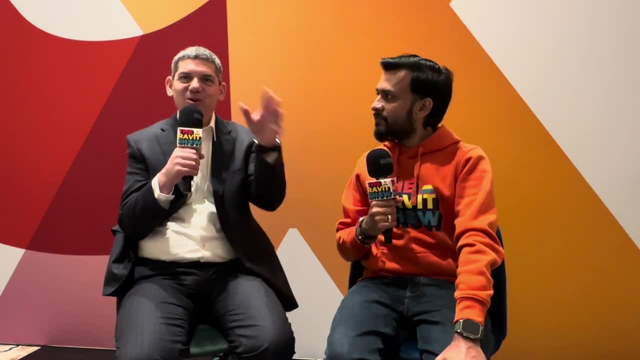 to GemIIni training to then kind of get that back right, That closed loop of influence on how we're training. the model is how we're improving systems for customers. I think Google is in a very special place in the industry: right to be able to serve our customers better. 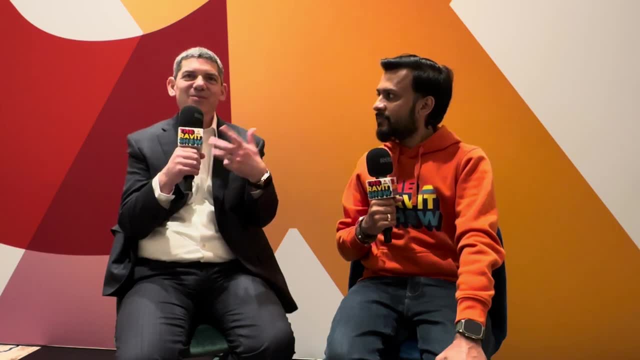 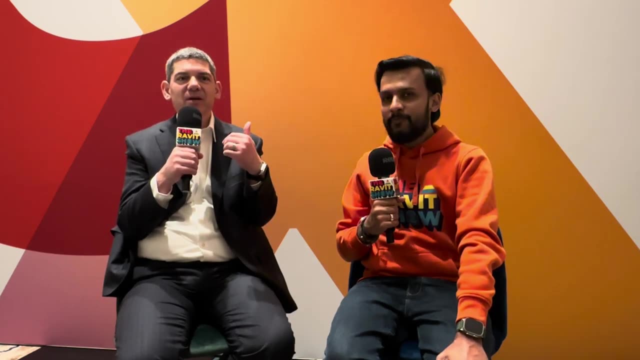 So that's been very exciting to us where the database team can actually make an impact on how we're training models. And then you know, as I said before, from our perspective, really two key opportunities to serve our customers better. One: innovative: 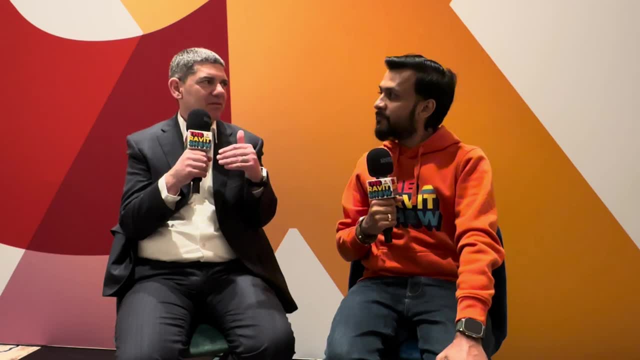 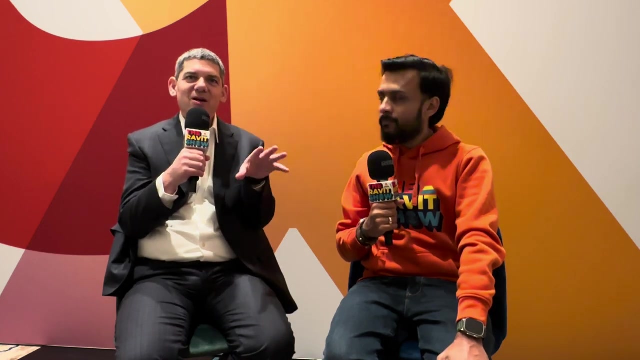 on core capabilities that databases have to make Gen-AI development easier, faster, more secure, more price performant. And this is where you're going to see things like vector support, ecosystem integrations, natural language support, security features all coming into the database And then 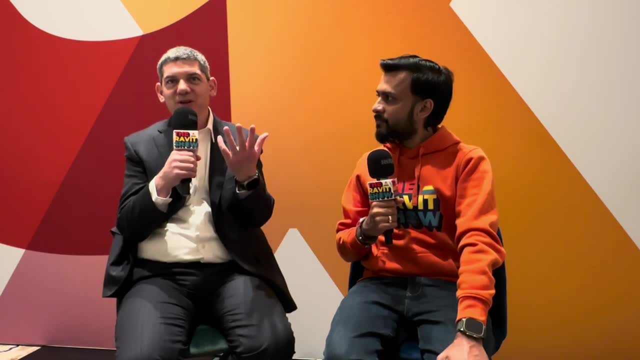 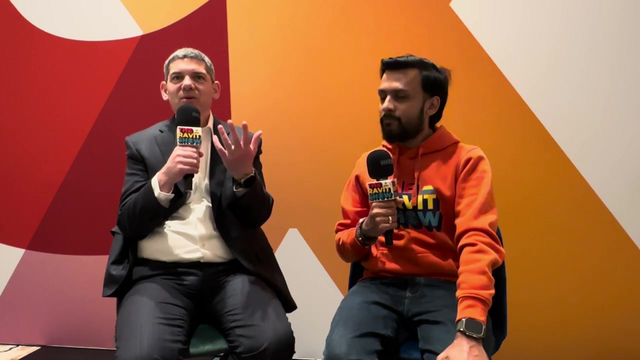 the second opportunity is: how do we use Gen-AI in Gemini databases to make our customers way more productive? And there's so much innovation we think we can deliver to make developers and operators really more productive And, frankly, what that means for businesses is they can take. 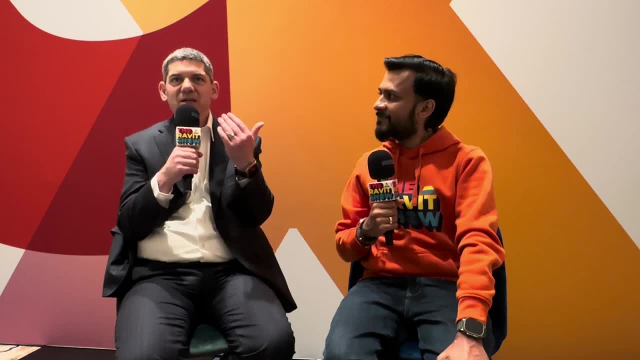 their highly valued staff and spend more of their time actually focused on business outcomes as opposed to taking care of the undifferentiated. you know heavy lifting of managing the infrastructure- Love it. Thanks for sharing those insights, And for anyone who's getting into AI, 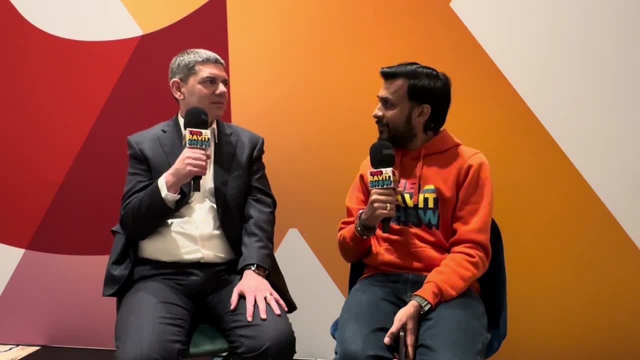 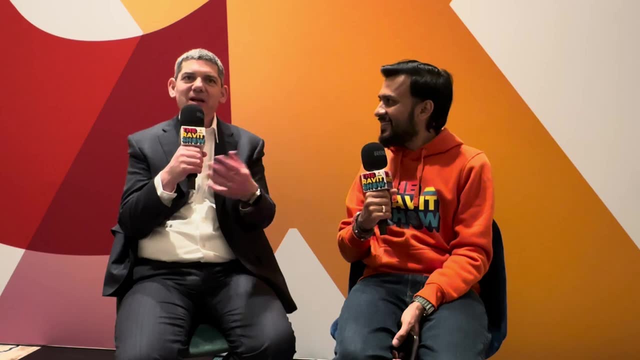 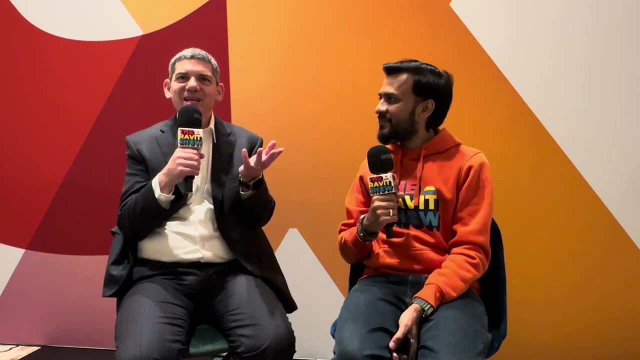 Gen-AI and building apps as well. do you have any advice for them, Any good practices, best practices that you would like to suggest? I mean this will sound self-serving, but I actually mean it. Download the LODB Omni. Start playing around with vector embeddings, because that's really the fuel of what. 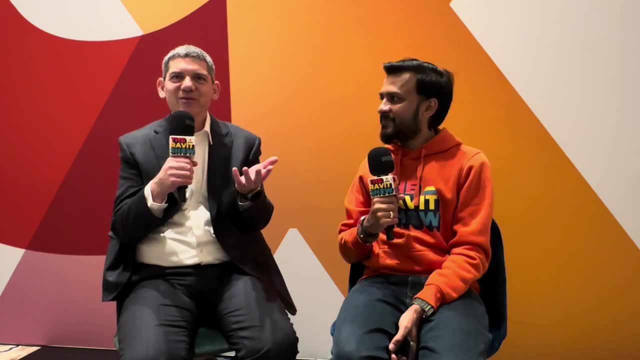 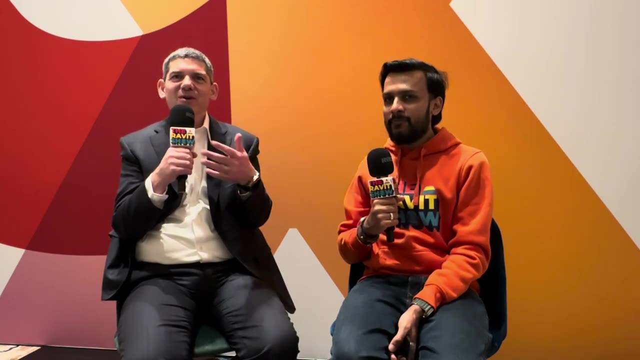 enables you to get the right prompts built for foundation models And just kind of experiment, whether these are, you know, embedding models on text or so on. We're just kind of running some similarities. I think you'll find very quickly by just playing around a bit in an environment that you kind of 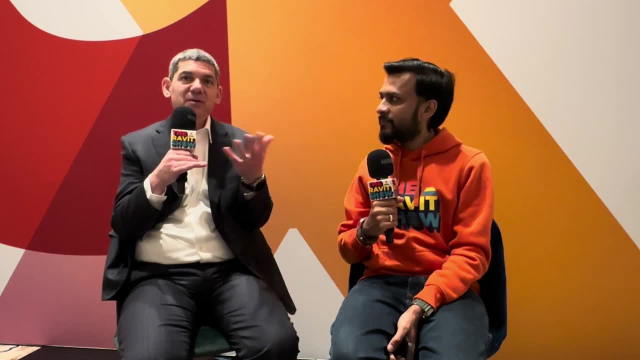 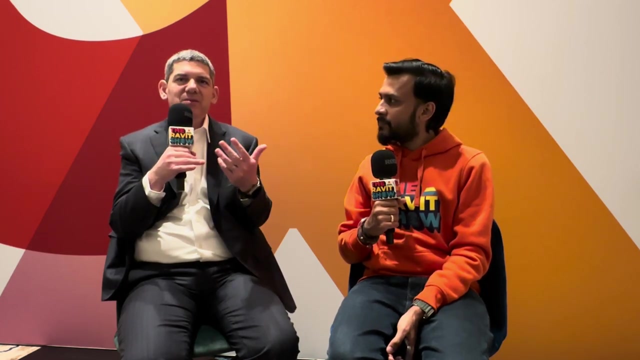 already know. like you know, 50% of database, 50% of developers are using Postgres, so it's a very familiar environment. I think you will very quickly see the power of you know what vector embeddings can do, how to start using foundation models And I think once you get kind of those first steps going, 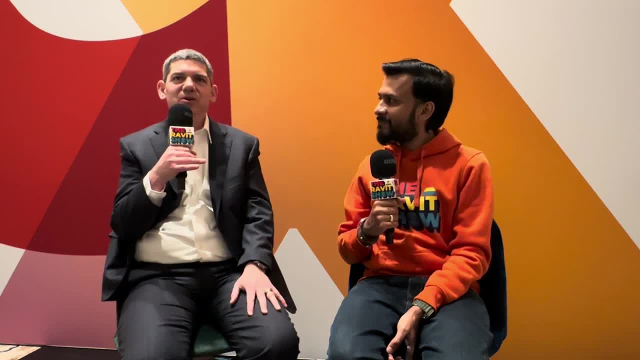 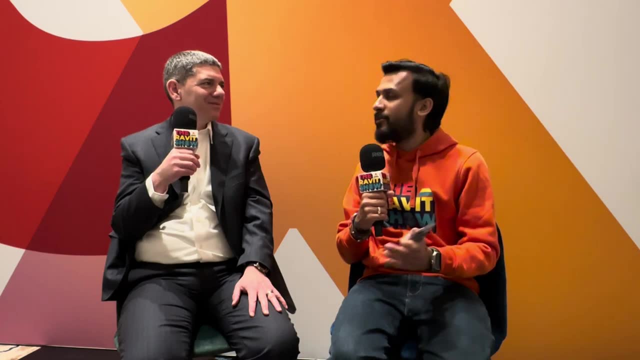 you know it's your Things happening almost automatically, But definitely in the end you can build up your imagination that really controls what you can build. Wow, I love it And thanks for sharing that. One last question for our audience. 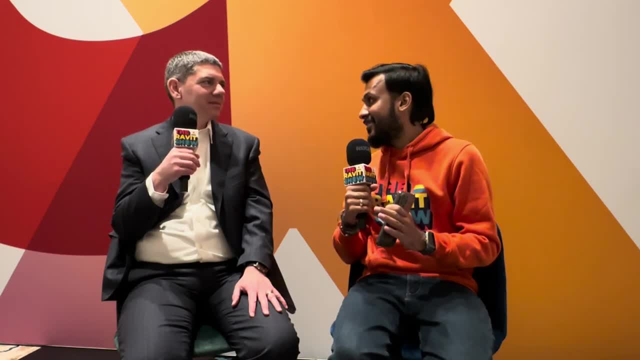 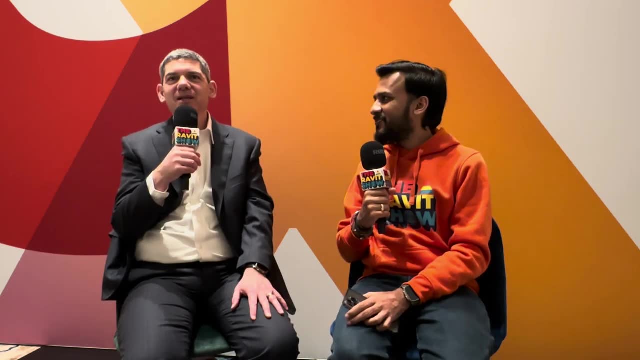 If folks want to reach out to you, if they want to follow the content. I follow you on LinkedIn, so I know the blog, the white papers that you put out at length. I love reading them, but any other place Or LinkedIn is the best place. 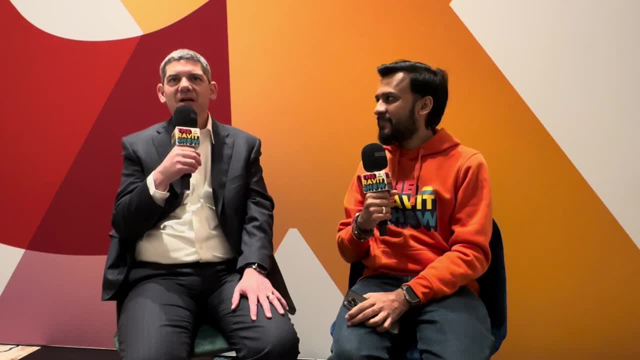 First of all, thanks a lot. You know I have mostly moved to using LinkedIn, So I would say that is that has become the best place to kind of get the latest around the database. You know services I lead and some my thoughts fantastic. Thank you very much for your time today. This was. 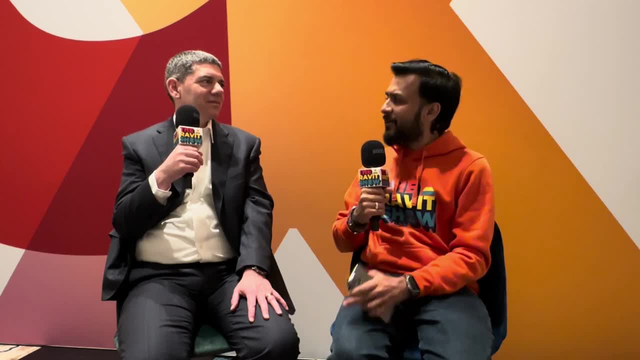 Amazing, great insights, Andy, and definitely looking forward to keep our conversation going, Thank you. Thank you everyone, Thanks.